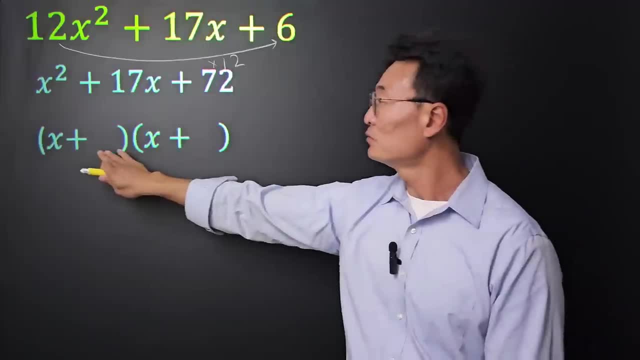 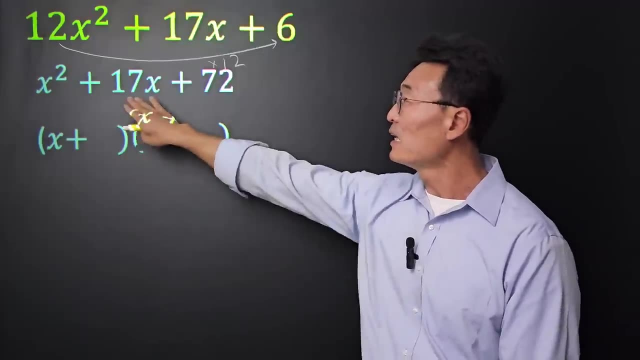 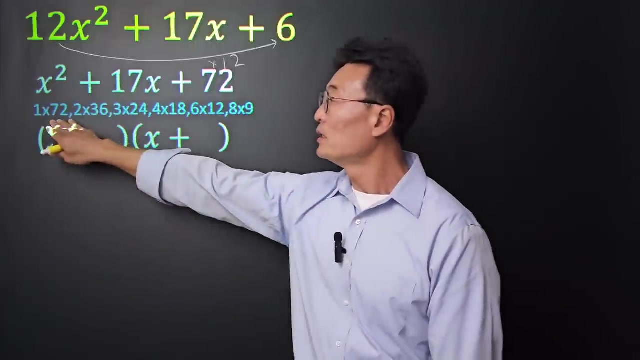 this. we have x plus and x plus, And to find out the two numbers that goes in here, we need to find two numbers: that multiplies to 72 and adds up to 17.. First of all, the list of numbers that multiplies to 72 are 1 and 72,, 2 and 36,, 3 and 24,, 4 and 18,, 6 and 27, and 8.. And we're going to 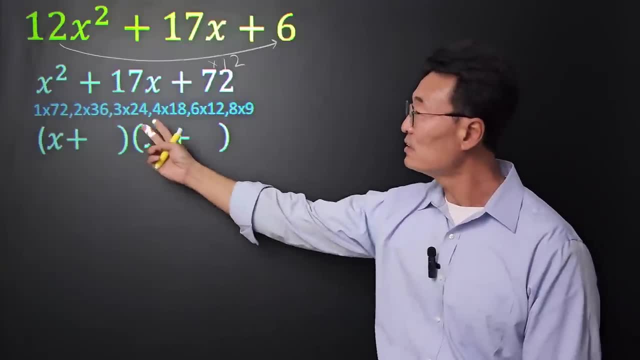 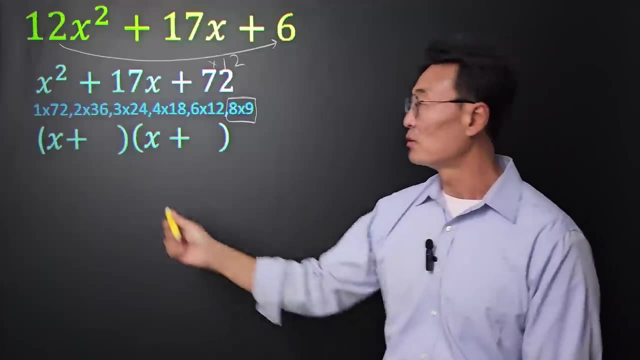 take 12 and 8 and 9.. Then, of these pairs of numbers that we have, what two numbers adds up to 17?? 8 and 9.. So I'm going to put 8 here and I'm going to put a 9 here Next. you know that 12, that 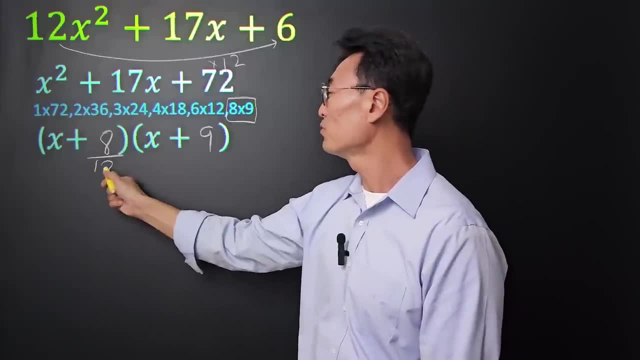 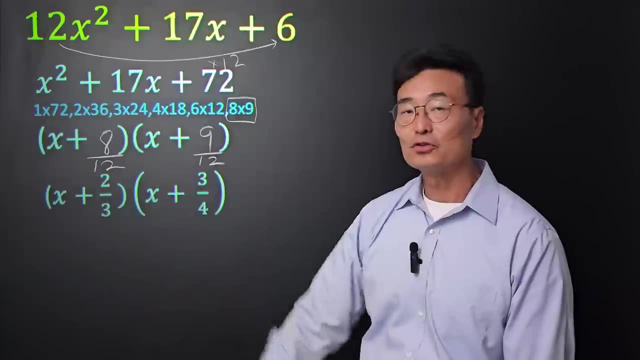 we multiplied. Where did it go? Well, we multiplied by 12, so I'm going to divide it by 12 here. Then, once we reduce the fractions, it becomes x plus 2 over 3, and x plus 12.. 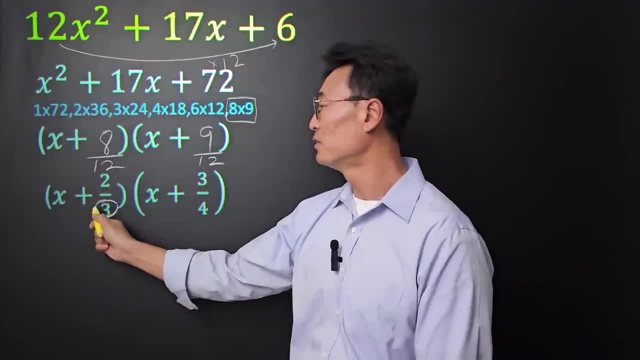 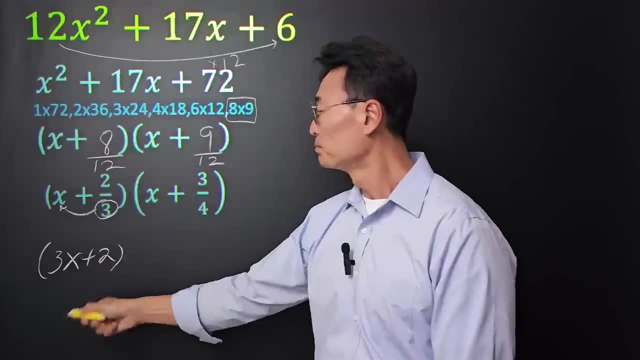 3 over 4.. To complete, all we have to do is take the denominator multiply to the x. Take the 3, multiply to the x, giving us 3x plus 2.. Next we're going to take that 4, multiply to the x. 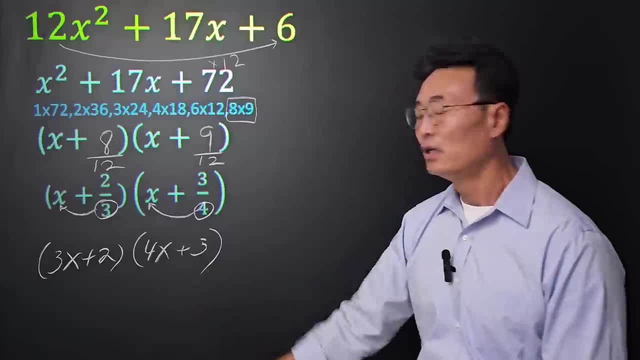 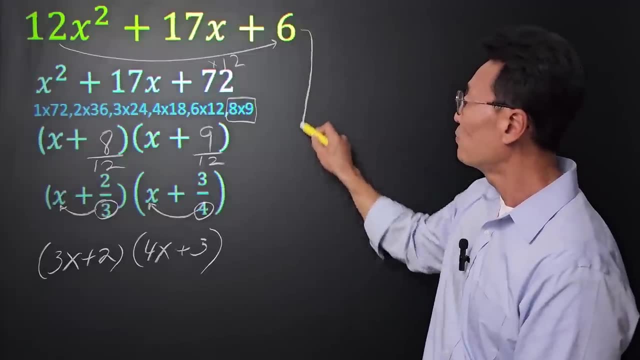 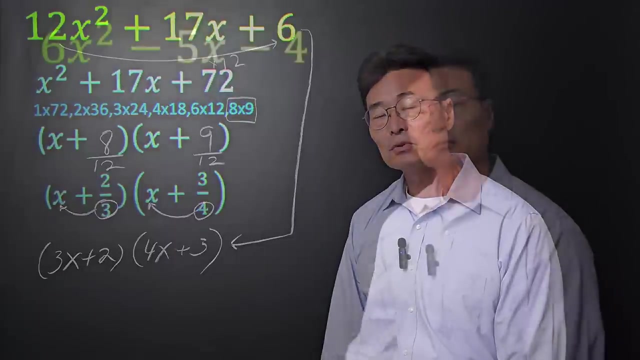 giving us 4x plus 3.. And, of course, if you multiply this out, you'll get 12x squared plus 17x plus 6, or factoring the original expression, that will be our final answer. Let me do another example. Here's the second example. Just as in the first example, I'm going 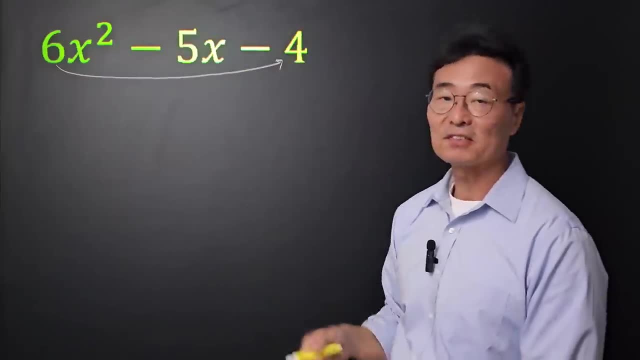 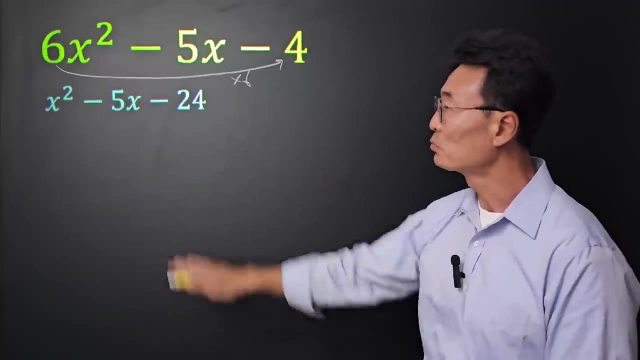 to take the leading coefficient, the 6, multiply to the c value, where we get x squared minus 5x minus 24.. Next we're going to factor this thing And again we get the x in the front. However, 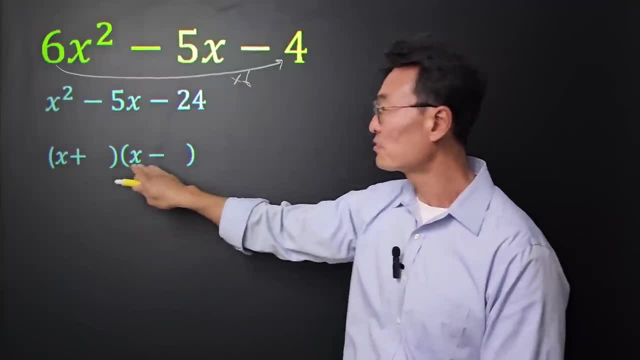 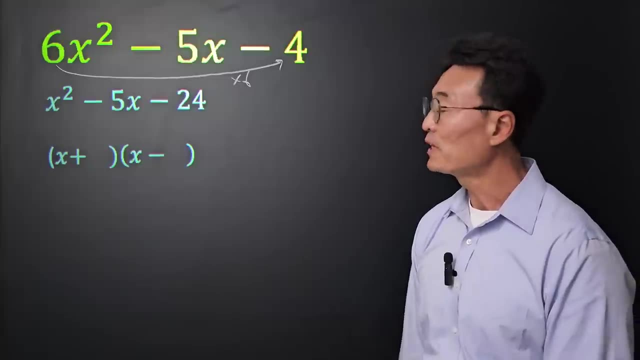 because this is negative. the third term it's going to be plus minus. Again. whenever the third term is negative, we get one plus and one minus. So we're going to take the leading coefficient. Again, we need to find two numbers that multiply to 24 first, which are 1 and 24,, 2 and 12,. 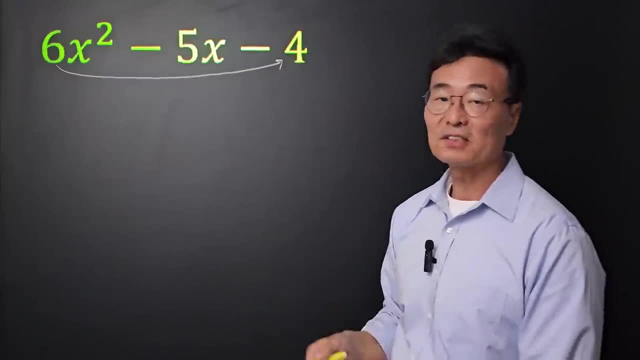 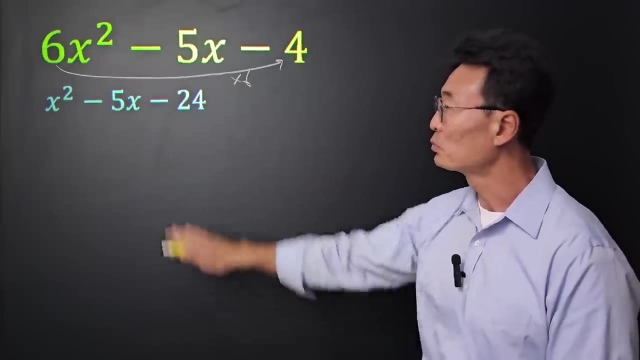 to take the leading coefficient, the 6, multiply to the c value, where we get x squared minus 5x minus 24.. Next we're going to factor this thing And again we get the x in the front. However, 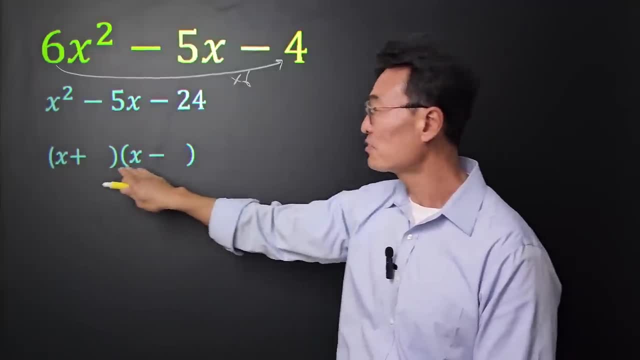 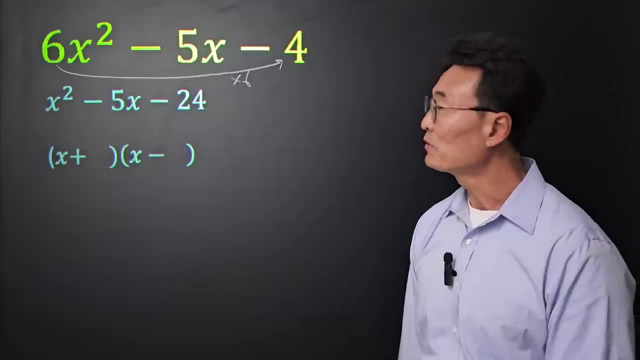 because this is negative. the 3rd term, it's going to be plus minus Again. whenever the 3rd term is negative, we get 1 plus and 1 minus Again. we need to find two numbers that multiply to 24 first, which are 1 and 24,, 2 and 12,. 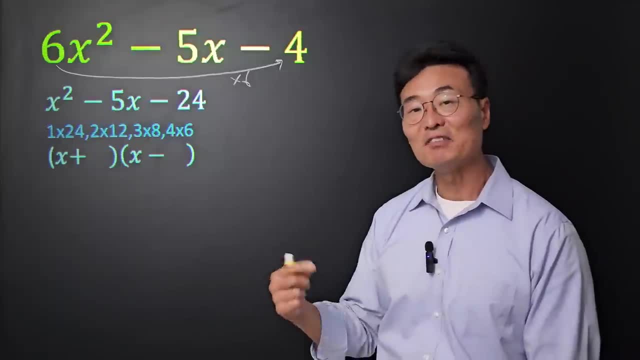 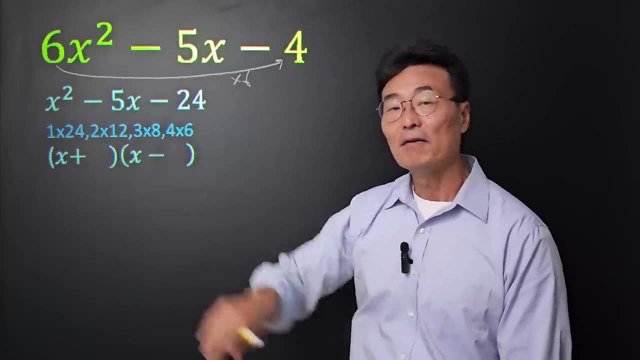 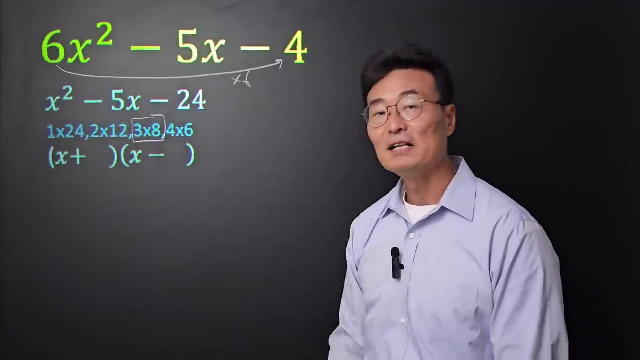 3 and 8,, 4 and 6.. And this time, instead of adding, because the two signs are opposite of each other, we want to find two numbers where we subtract and get 5. And it's going to be 3 and 8, because 8 minus 3,, of course, is 5.. 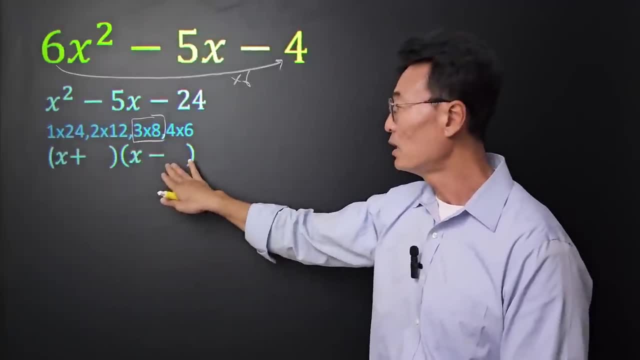 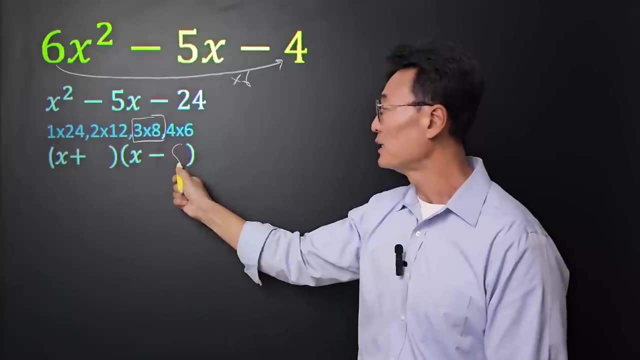 Only thing you have to figure out is: does the 8 go here? or the 8 goes here, Since it's negative- 5, we want to put the bigger number with the negative, so we put the 8 here, and the other number, or the 3, goes right there. 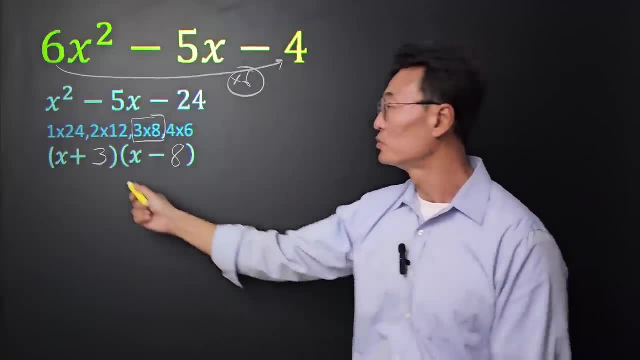 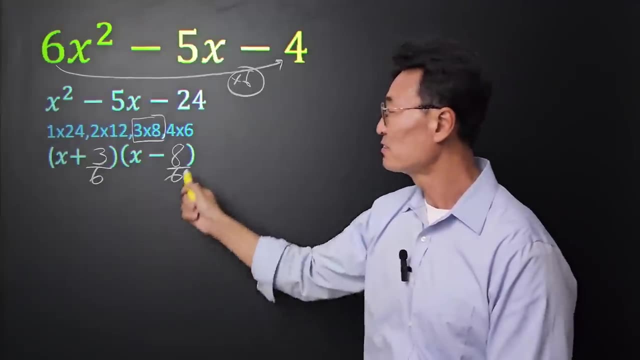 Next, here's that 6 that we multiplied. I'm going to divide the 3 and the 8 by 6. And by reducing the 3 over 6 and the 8 over 6, we get x plus 1 half. 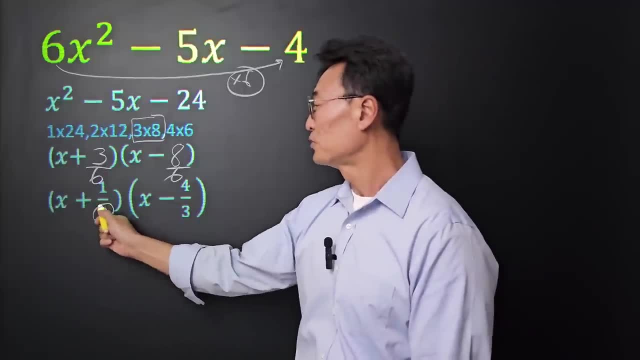 And x plus 2. And x plus 1 half And x plus 1 half, x minus 4 over 3.. We're going to take that 2, multiply to the x, giving us 2x plus 1.. 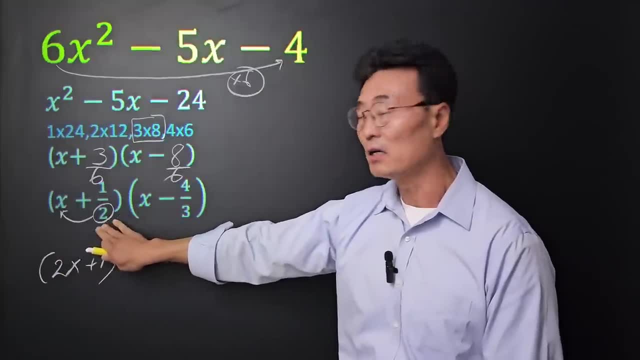 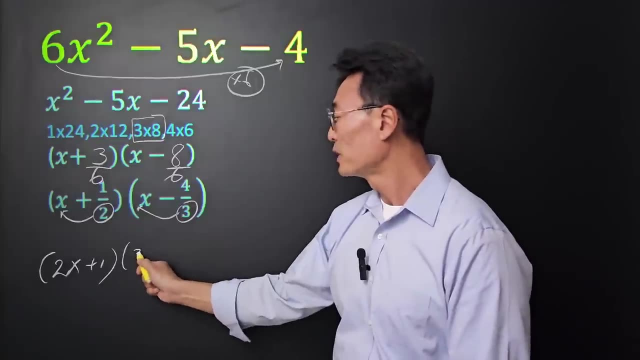 Notice: the 1 stays. the 2 is gone since we packed it onto the x. Again, we're going to take that 3, pack it onto the x or multiply where we get 3x minus 4.. Again, if you multiply this out, 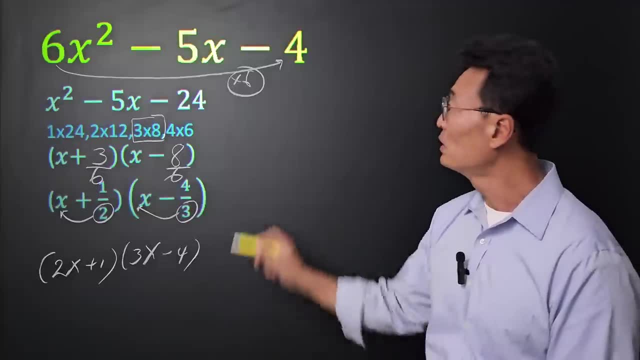 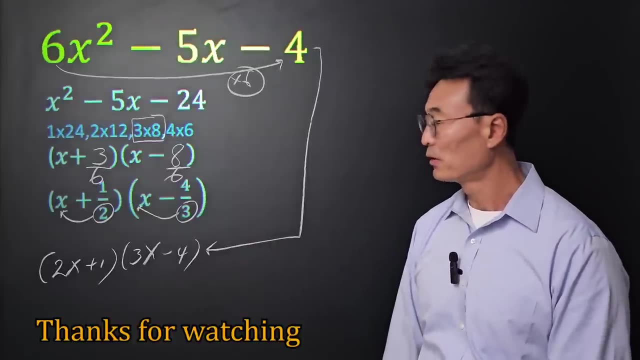 you'll get 6x squared minus 5x minus 4, or if you factor the original expression, the trinomial, once again, we get 2x plus 1, 3x minus 4.. So I hope this method, if you haven't. 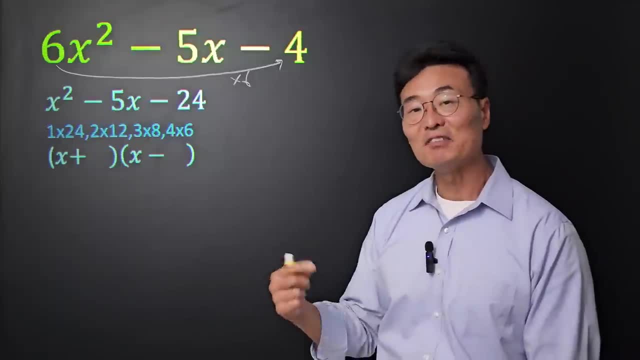 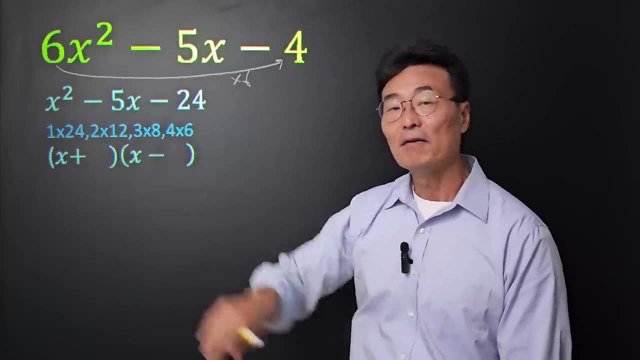 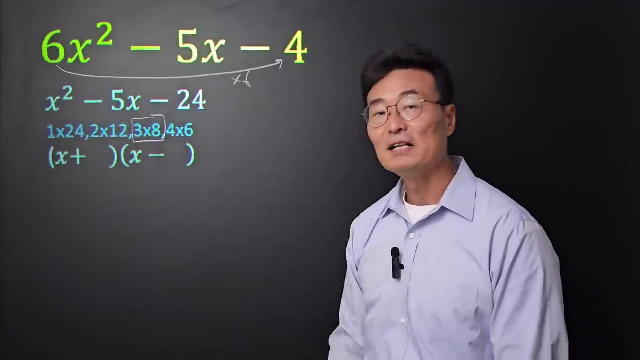 3 and 8,, 4 and 6.. And this time, instead of adding, because the two signs are opposite of each other, we want to find two numbers where we subtract and get 5. And it's going to be 3 and 8, because 8 minus 3,, of course, is 5.. 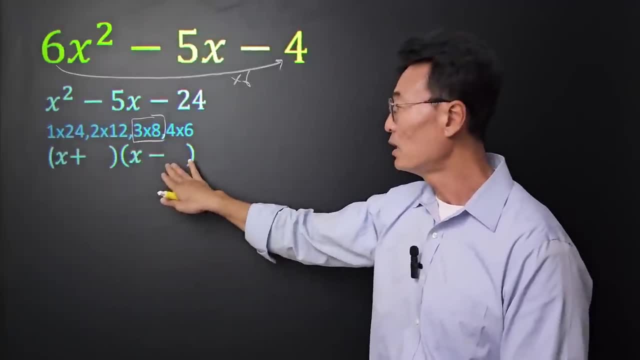 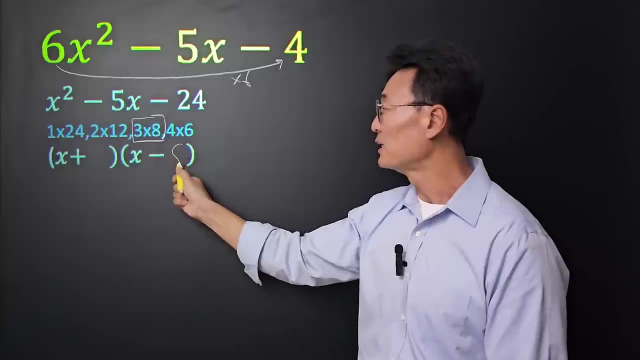 Only thing you have to figure out is: does the 8 go here? Or the 8 goes here, Since it's negative- 5, we want to put the bigger number with the negative, So we put the 8 here and the other number, or the 3, goes right there. 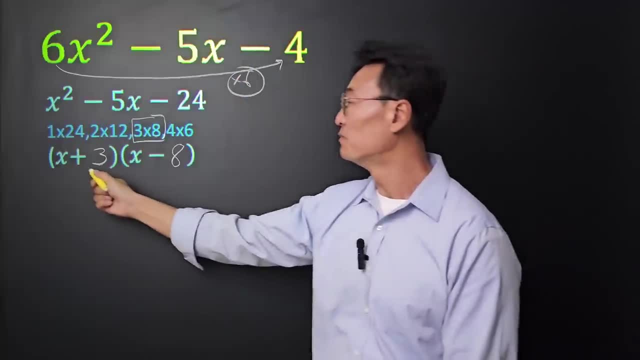 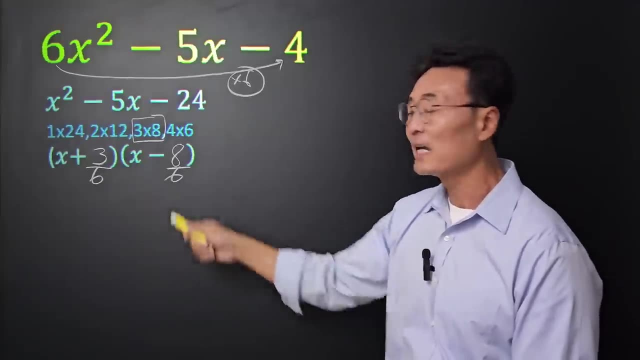 Next here, with that 6 that we multiplied, I'm going to divide the 3 and the 8 by 6. And by reducing the 3 over 6 and the 8 over 6, we get x plus 1 half. 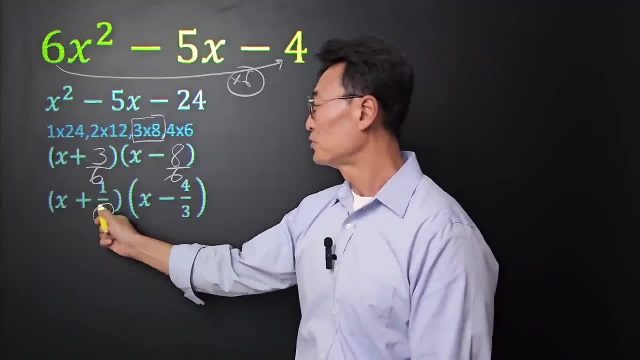 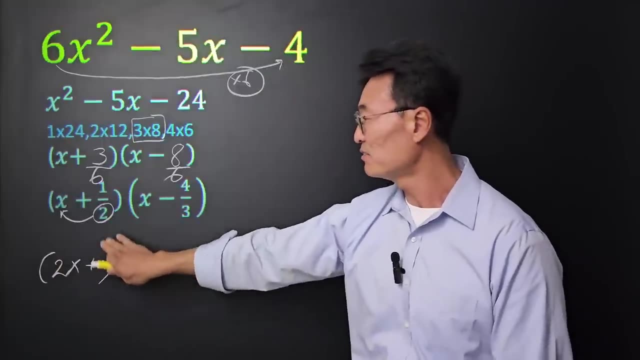 And x minus 1.. x minus 4 over 3.. We're going to take that 2, multiply to the x, giving us 2x plus 1.. Notice, the 1 stays. the 2 is gone since we packed it onto the x. Again, we're going to take that 3,. 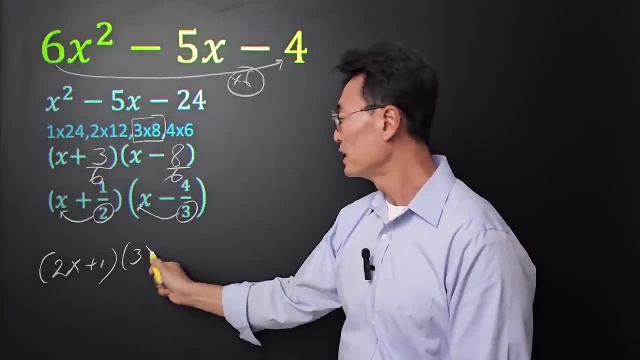 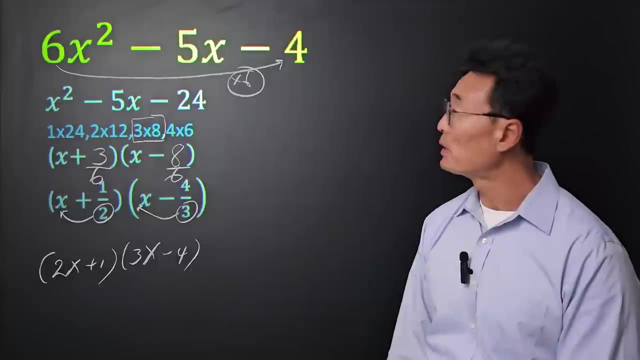 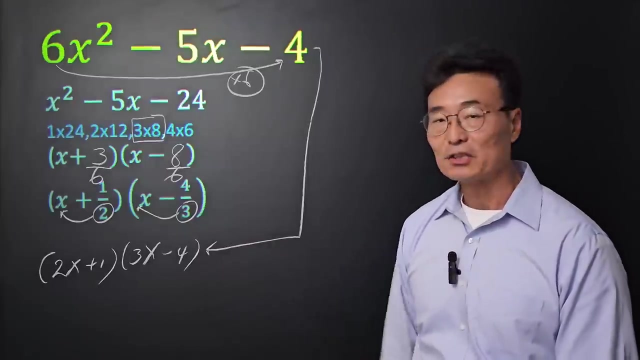 pack it onto the x or multiply where we get 3x minus 4.. Again, if you multiply this out, you'll get 6x squared minus 5x minus 4, or if you factor the original expression, the trinomial, once again we get 2x plus 1, 3x minus 4.. So I hope this method, if you haven't, 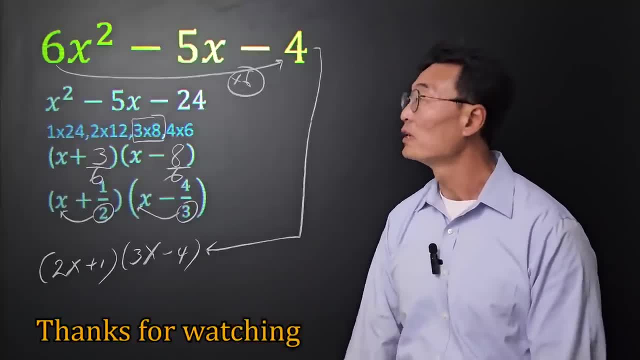 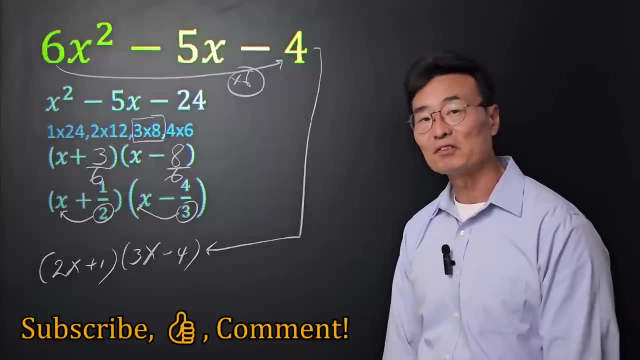 seen it before- will help you factor trinomials with a leading coefficient other than 1.. As always, thank you very much for watching my videos and supporting. If you haven't subscribed, please do so and give it a thumbs up. Thank you.